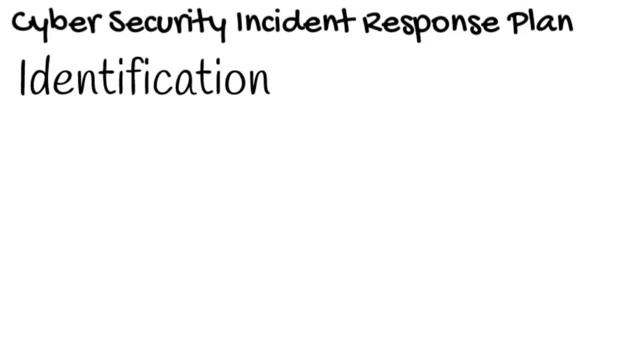 Having an adequate setup is paramount to the ability to identify that an incident has occurred. This is usually where alerts from intrusion detection systems come up. Web filtering gateways detect a suspicious external connection. SIEM solutions connect the dots of an attacker passing through the internal network. This is usually the first step in the process of 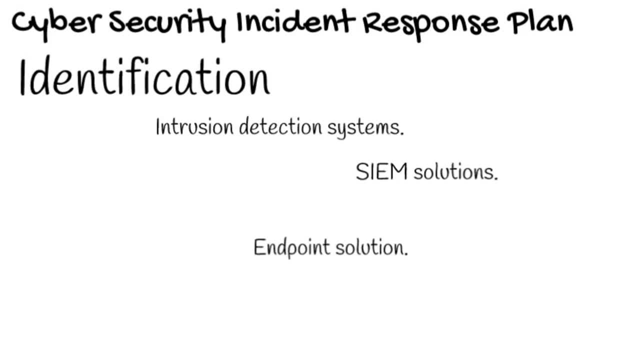 identifying an incident. 2. Identification is the first step in the process of identifying an incident. 3. Identification is the first step in the process of identifying an incident. A whatnot Onder wichtige Anекov 25 or an endpoint solution. alerting of a phishing email opened, No matter the 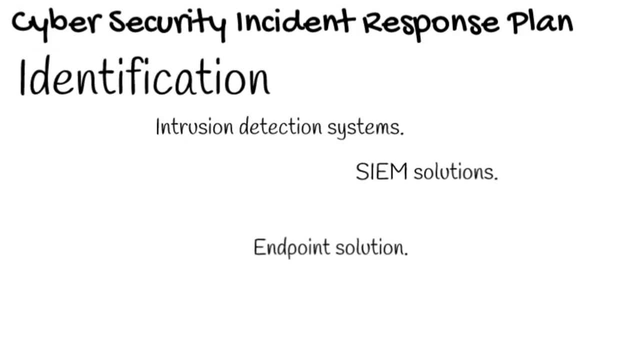 case, quick reaction from qualified security staff is needed in order to escalate and respond to the alerts. 3. Containment: This is the third stage of the CRP lifecycle In order to stop further spreading of malware and damage to the network and data theft. containment of the threat actors is what 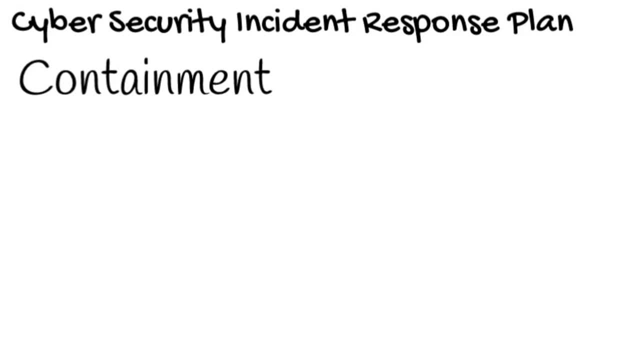 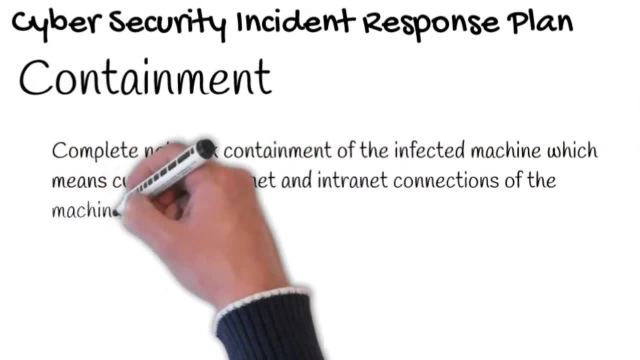 is needed in order to focus on the next stage of the incident response. A good example in practice would be a complete network containment of a Java location in the home underground of the infected machine, which means cutting all internet and intranet connections of the. 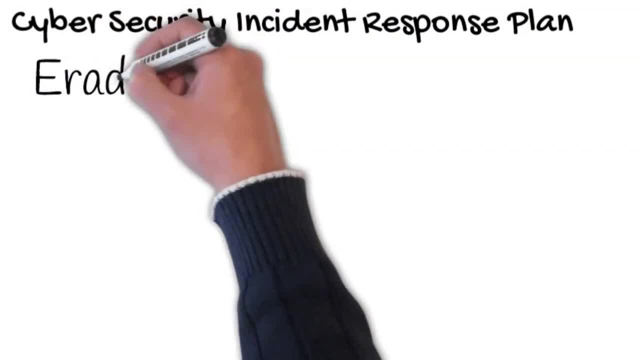 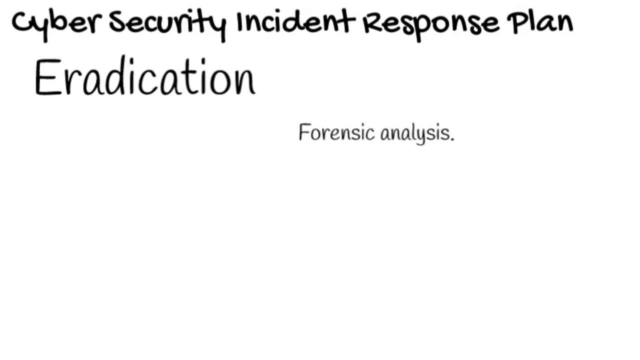 machine 4.. Eradication is one of the most complex stages in the incident process, as it involves forensic analysis in order to determine the extent of presence of the threat actor. Security staff need to make sure that what they do in the eradication stage eliminates 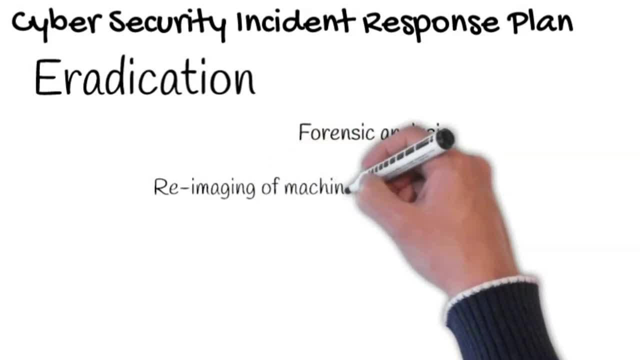 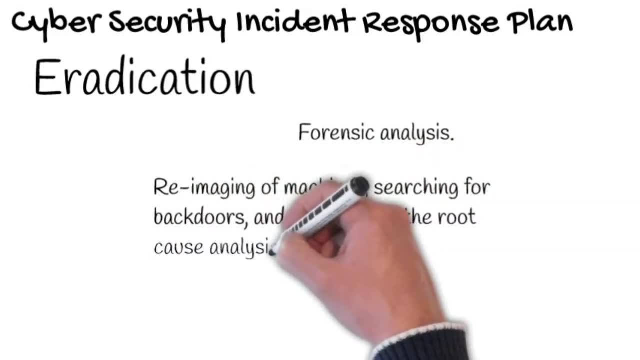 all presence and access of the threat actor to the system. This includes re-imaging of machines, searching for backdoors and, most importantly, determining the root cause. analysis of the incident Depending on the root cause eradication stage can be simplified by knowing the vector of. 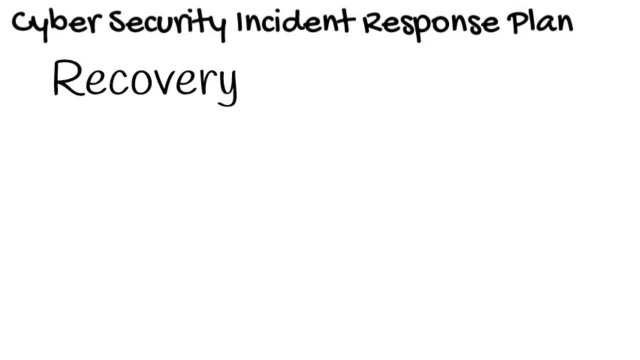 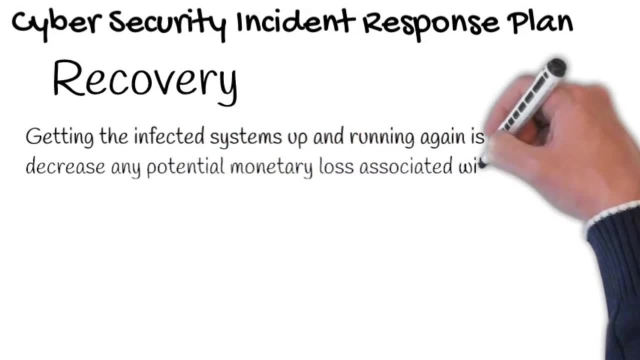 attack that took place. 5. Recovery stage comes right after eradication. In this stage, getting the infected systems up and running again is important to decrease any potential monetary loss associated with the downtime of the infected system. In some cases, a single computer infected with a virus is not going to bring down the 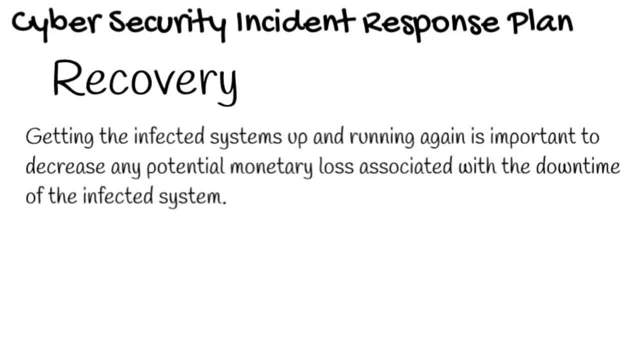 company, but an office with 100 employees whose computers fell victim to ransomware is a whole other story. In the later case, quick action from the CPU Security team will determine how big the loss of revenue will be. Also, lessons learned is one of the most important stages, for a simple fact that it will showcase.